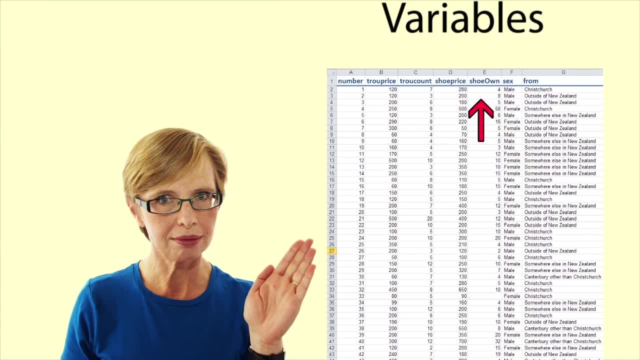 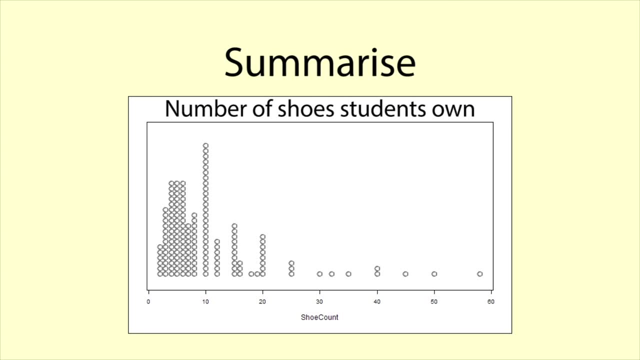 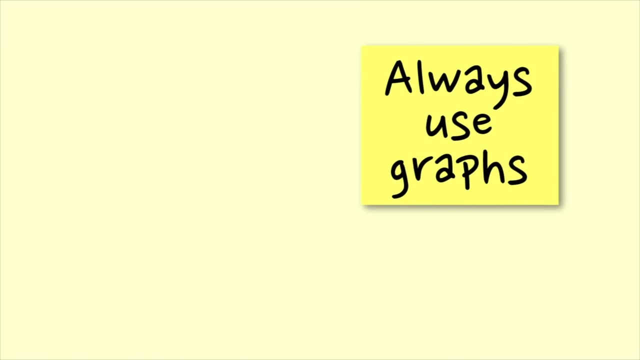 A data set is made up of variables and observations. We may want to summarise the distribution of values for each of the variables. Often, we wish to compare two groups within a set of data. We should always use graphs to explore and analyse the data. You can see how. 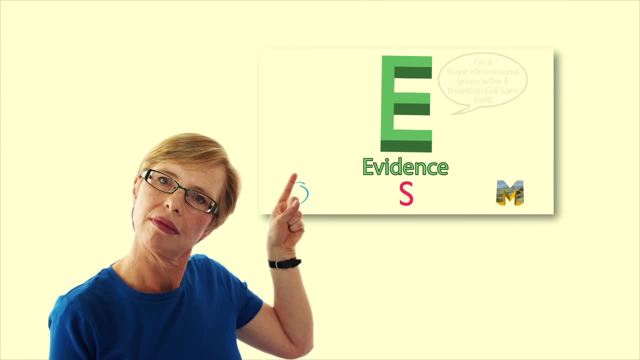 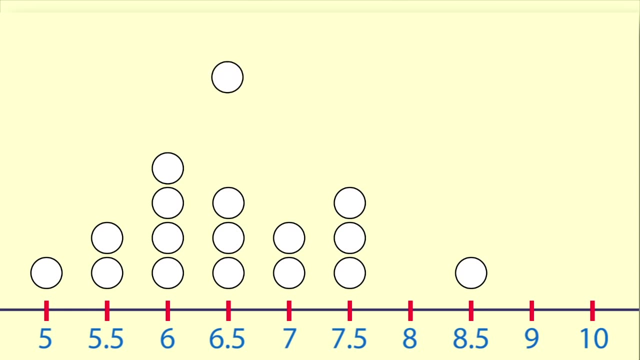 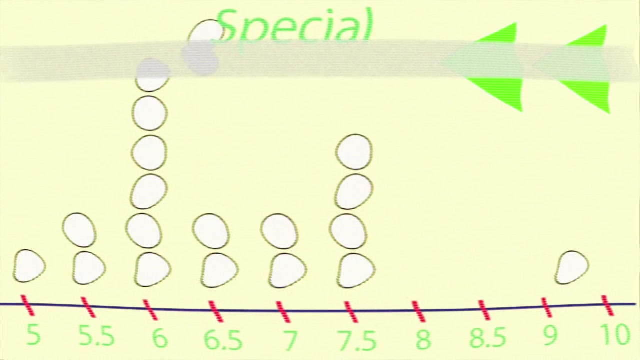 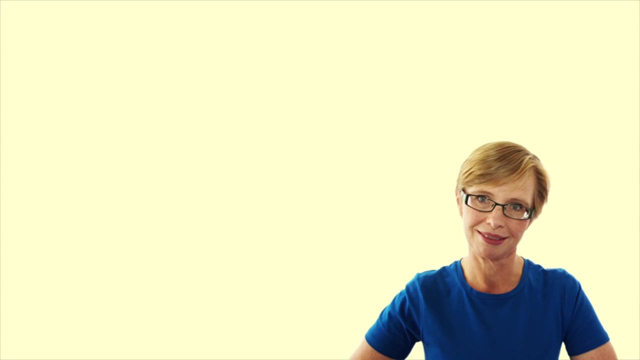 to do this in our video analysing and commenting on graphical output using OSIM. When we explore data, we are interested in position, spread, shape and special. In this video, we will mainly talk about position. To summarise the position or location of the data, we use the mode median or mean. 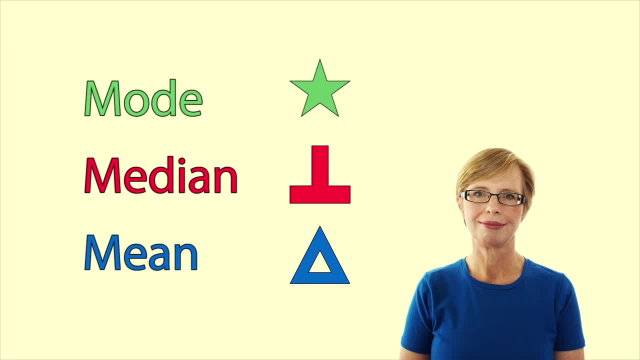 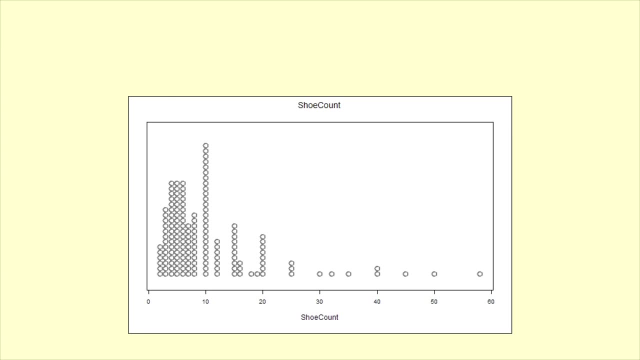 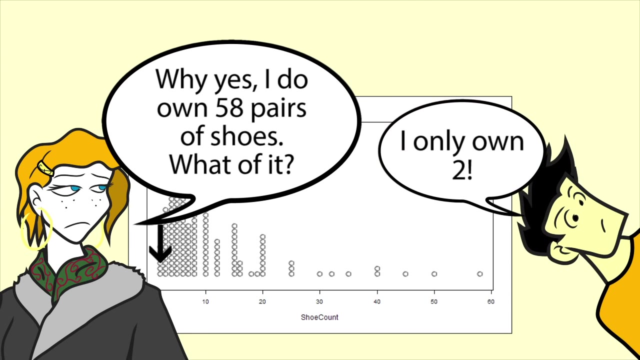 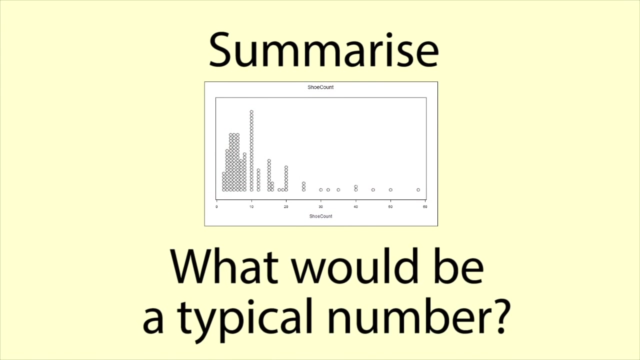 We will illustrate this with an example. Here is a dot plot of the number of pairs of shoes 161 students said that they owned. Each dot corresponds to one person and indicates how many pairs of shoes that person said they owned. When we summarise, we look at the overall distribution and ask what would be a typical. 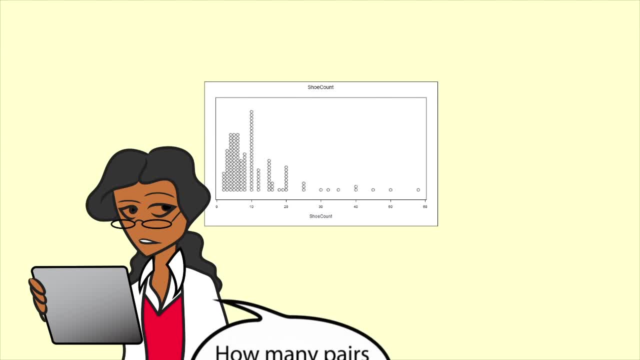 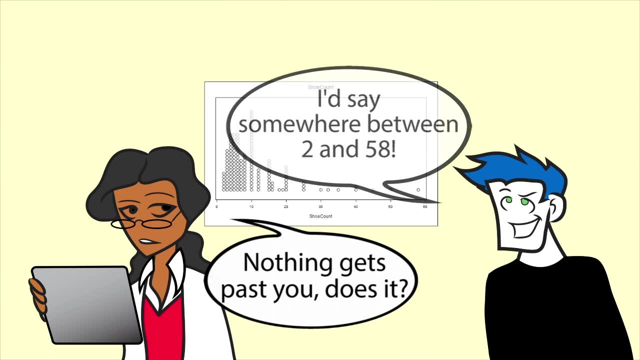 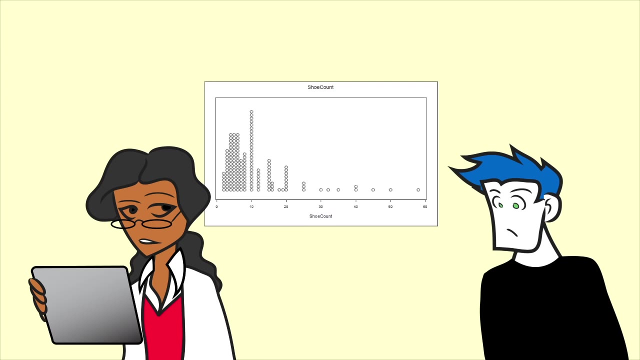 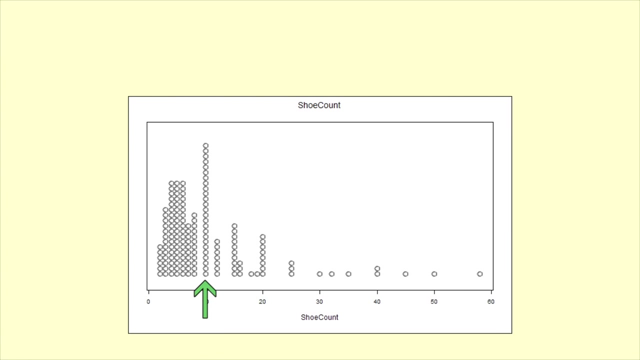 number. If someone asked you: how many pairs of shoes do these students own, There are several possible answers. For now, we are only going to allow a one number answer, a single indication of position or location. 10 is one possible answer. 25 people said that they owned 10 pairs of shoes. 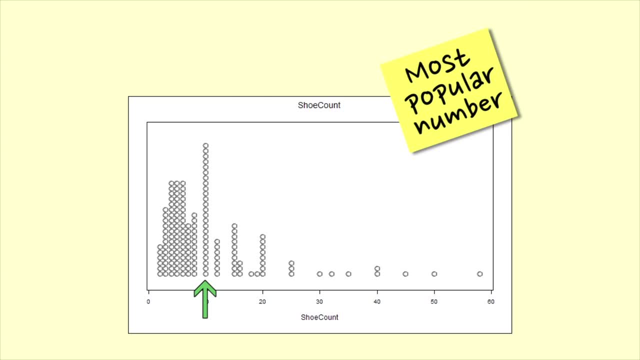 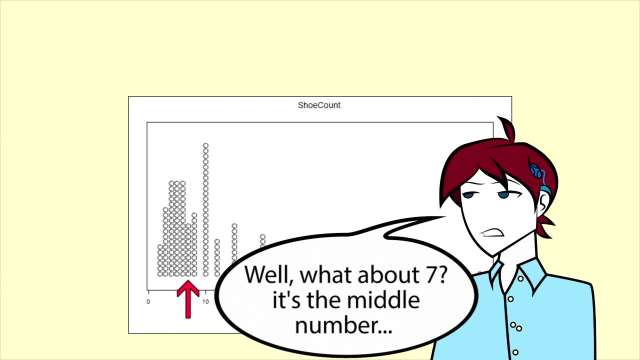 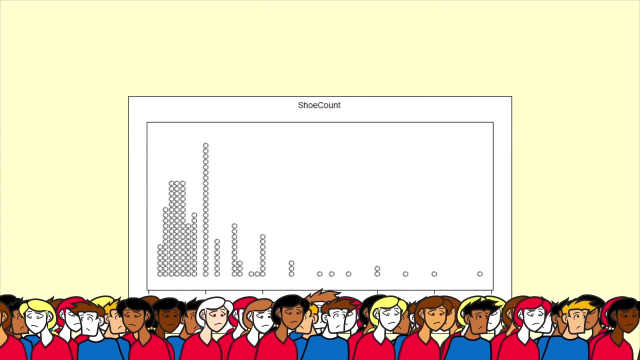 More people said they had 10 pairs of shoes than any other number. This is called the mode. Another possible answer is 7.. It is the number in the middle of the distribution. It is called the median. There are 161 students represented in our data set, so half way is student number 81.. 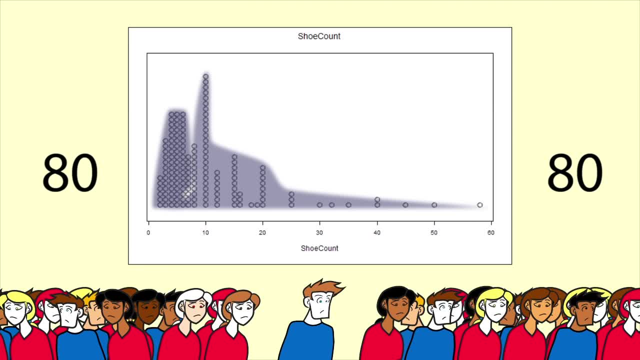 There are 80 students above and 80 below. That student in 81st place said he or she had 7 pairs of shoes, so the median is 7.. The other summary value is often called the average, though the more technical term is the mean. 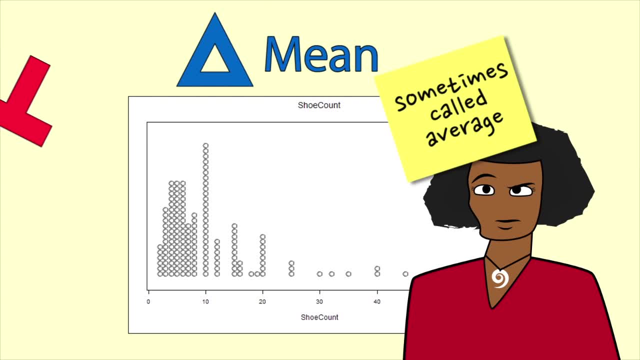 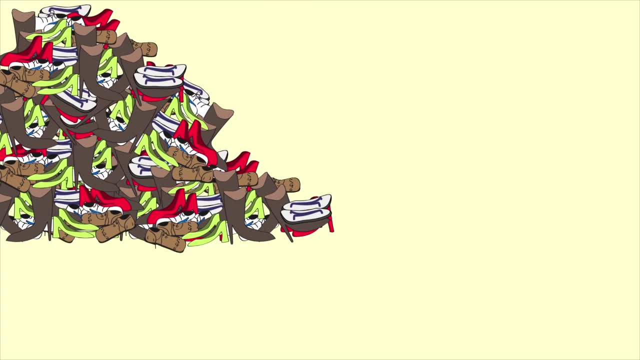 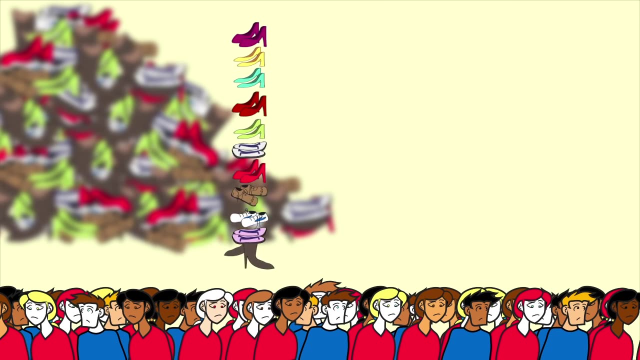 Sometimes average refers to the median, so it is safer to use the term mean. If we piled all the pairs of shoes together and distributed them evenly over the 161 students, they would end up with 10.07 pairs each. The mean number of pairs of shoes per student is 10.07.. 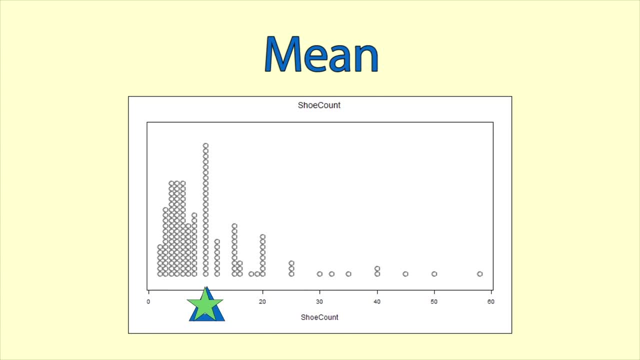 In this case, the mean is close to the mode, but this is only sometimes. For this set of data, the mean is quite a lot higher than the median. That is because there are a few people who own a whole lot of shoes. When their shoes are spread around, they cause the mean number of shoes per person to go up. 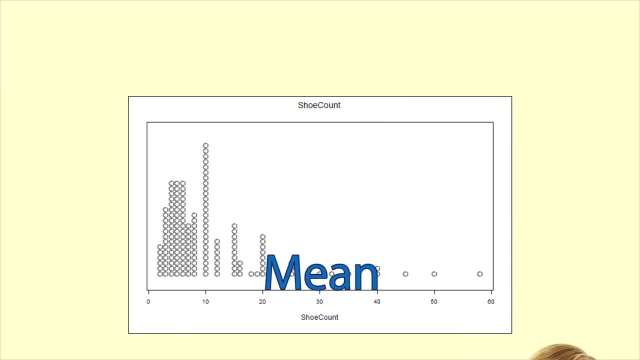 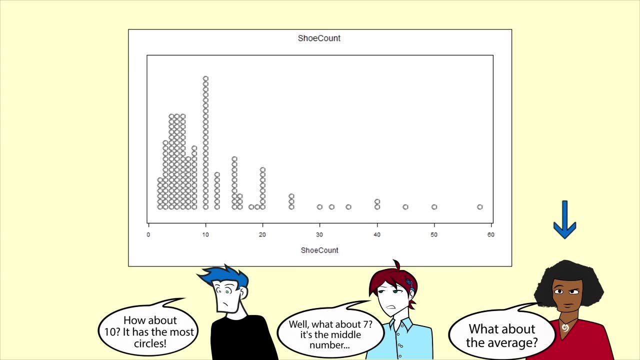 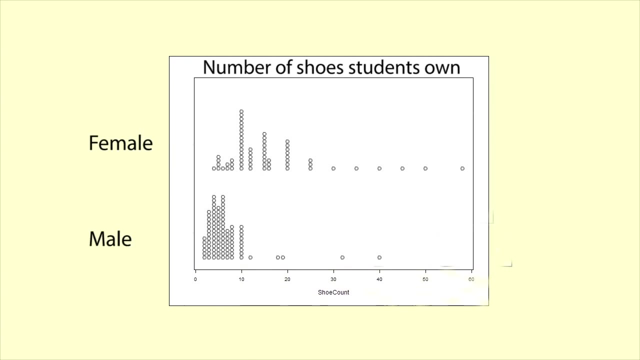 We will talk more about this later. When we report statistics, we need to decide which summary values are most indicative of the distribution of the data. To illustrate this, let's have a look at what happens when we separate out the students into female and male. 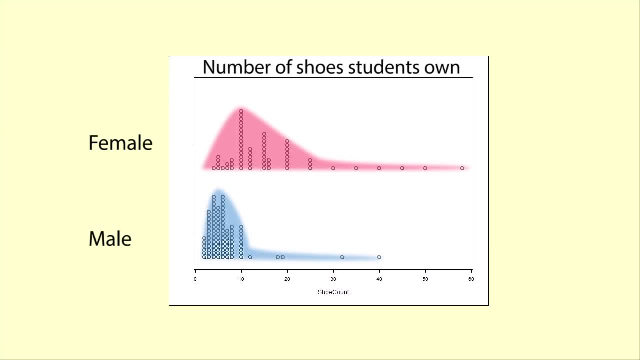 You can see that the two distributions look quite different from each other. For the female students, the mode is 10,, the median is 12, and the mean is 15.73.. For the male students, there are two popular values: 4 and 6.. There is no mode. 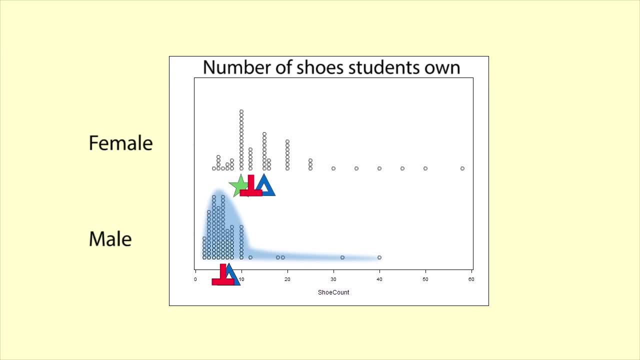 The median is 5, and the mean is 6.. In both cases, there are just a few people who have a whole lot more shoes than the others. If those extreme values weren't there, the means would drop to 12.86 and 5.8,, which are closer to the medians. 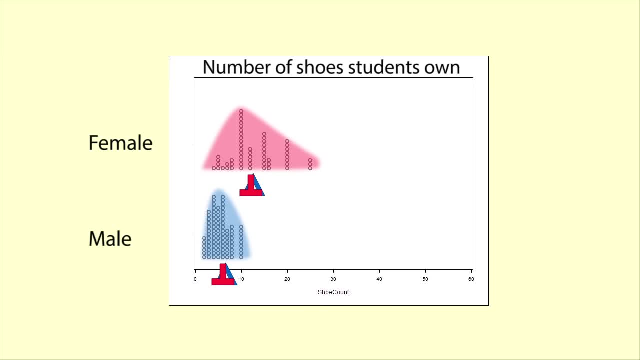 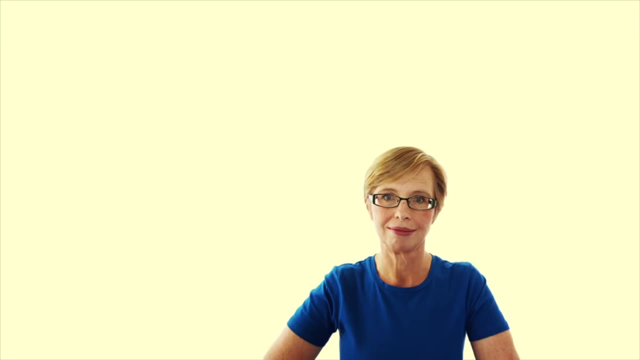 In both cases, when we remove the extreme values, the median does not change. In these examples, the median gives a better indication of the position or location of the distribution. The median does not change When you summarize the location or position of the data. 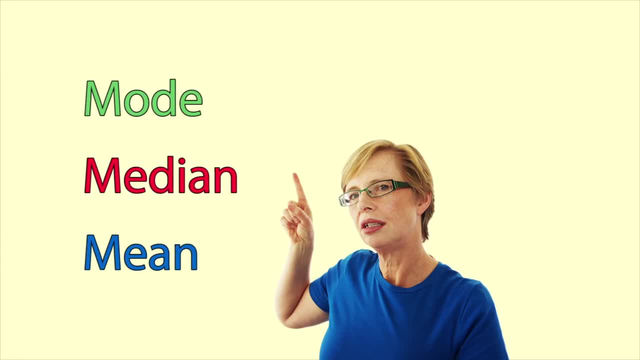 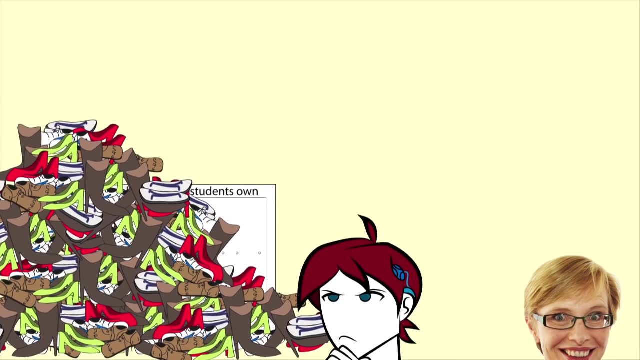 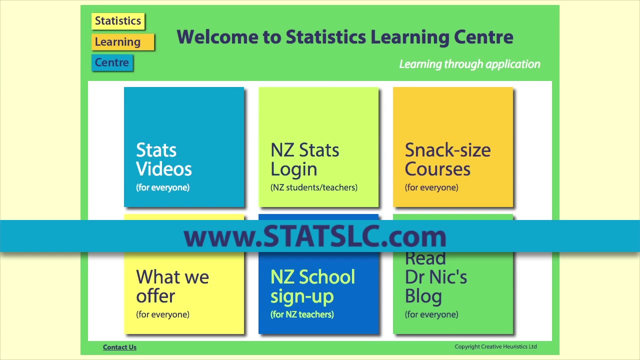 you will need to decide which is the most appropriate statistic. You need to look at a graph of the data and think about the context in order to make this decision. This video was brought to you by Statistics Learning Centre. Visit our website for more resources to help you learn.